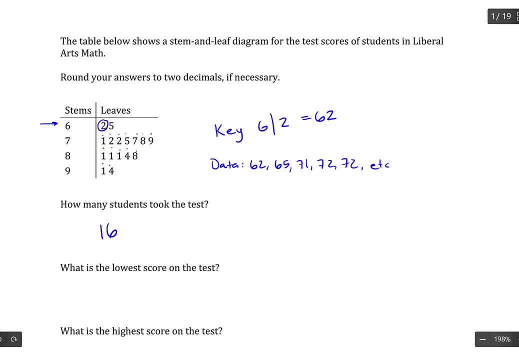 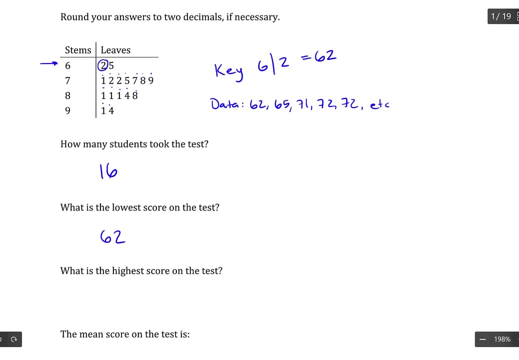 because that's going to be the lowest ones place. So a stem of 6 and a leaf of 2 gives me the lowest score of 62.. What is the highest score on the test? Well, we just do the opposite here. We just come down to the largest stem. 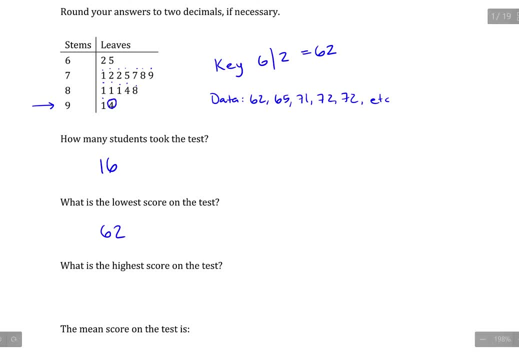 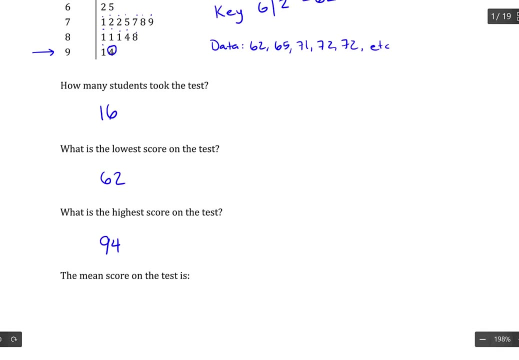 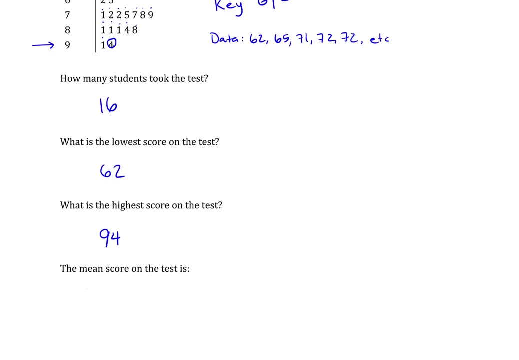 and the largest leaf within that stem represents the value that was the largest on the test altogether, The mean score on the test. Well, to get the mean of any data set, we take each item in the data set and add them together. So that's what's meant by this symbol, right here. 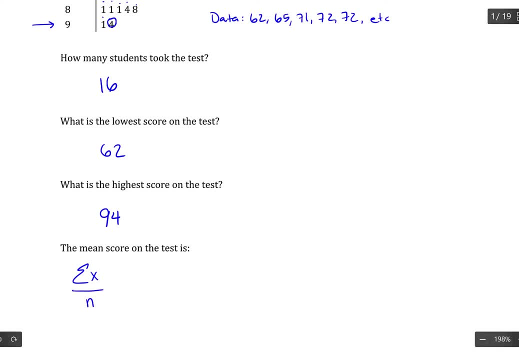 the sum of all the items in the data set And then we divide by the number of items in the data set and that gives us our mean. So we can use the calculator to help out. You can either take advantage of advanced features. 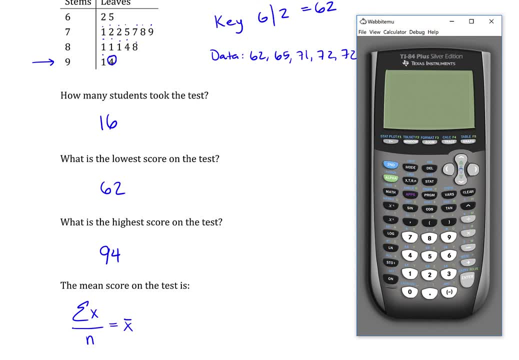 or since all we need is the mean of a small set of data, I think it's fine to just start typing in the data one item at a time, So 62 plus 65 plus 71 plus 72. And we just go through the data set until we have it all typed in. 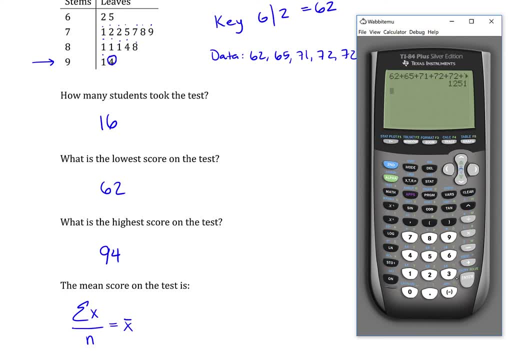 All right And we get the sum of all the data And then we have to divide by the number of data items that existed. So if I take that and divide it by 16, that gives me the mean score here, which, in this case, to two decimal places, I'll use. 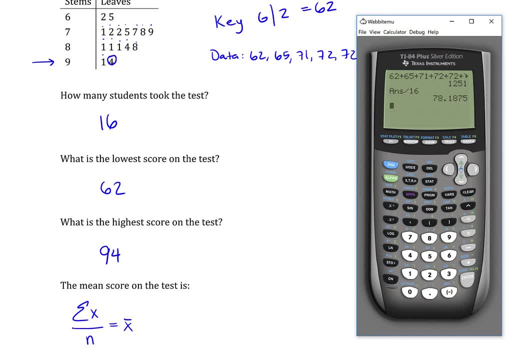 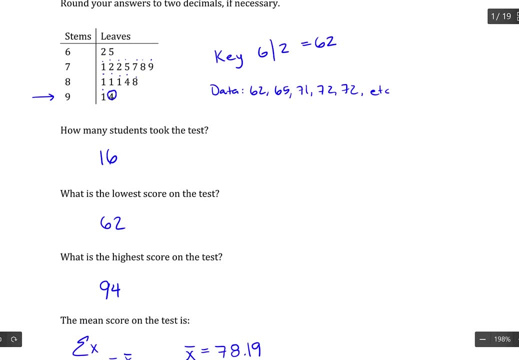 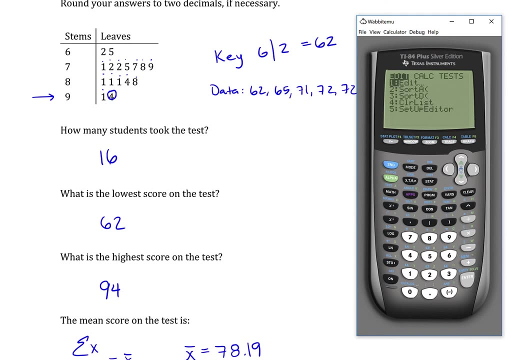 So 78.19.. So the mean of this data set is 78.19.. Now, if you're using more advanced technology, a lot of calculators have what's called a list editor, where you can edit a set of data at a time. 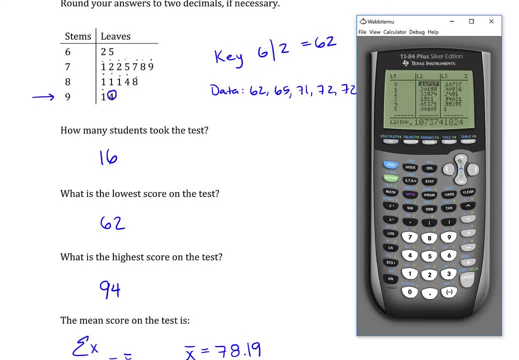 So if I hit Stat and then Edit, I can clear out some stuff that's already in here, And it works similar to a spreadsheet in that I can just type in each item one at a time. Now there's probably not going to be a time savings. 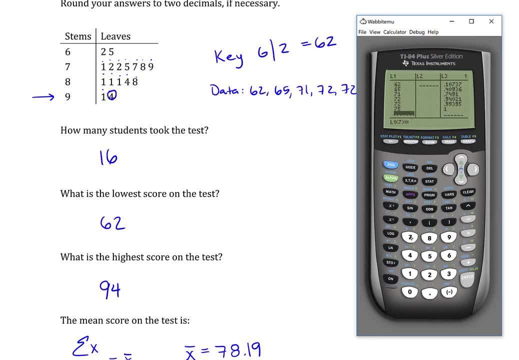 because, just getting the mean of this data set, I still have to type them in. It's not going to save me there, But it could save me from typing in a value incorrectly because I can scroll back up through the list after I'm done. 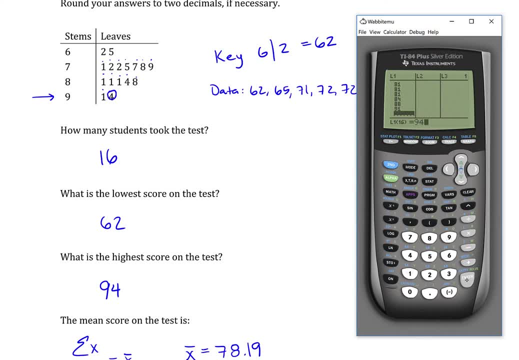 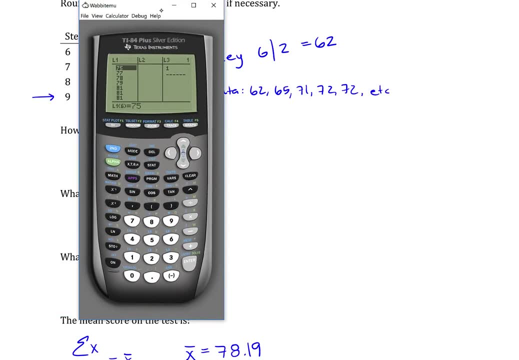 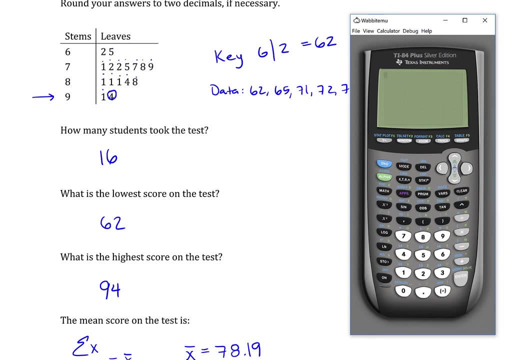 and double check all of my items. So it's a little bit safer, using a list editor, to enter all the data and then calculate from the list. Now, there's different ways we can do this. One way is you can do different list calculations. 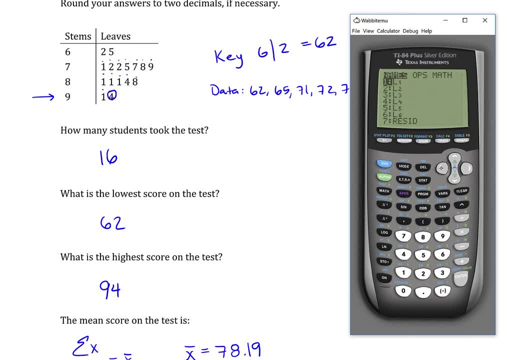 if you hit 2nd and Stat, which gives you list values, There's some different operations that can be done. You can come over here to Math and that's where your basic stats are, And the third one down here is the mean. 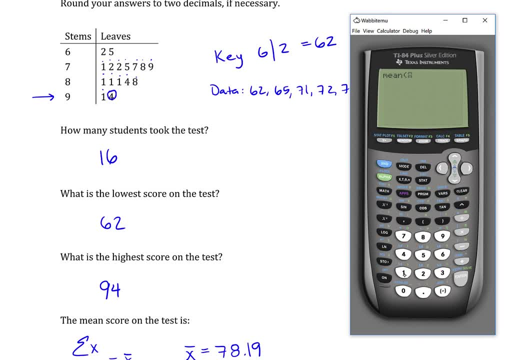 And you just need to tell it what list you want to calculate the mean of. So just hit 2nd and 1, and that will give it L1. And then it knows to add all that data together and divide by the number of items. 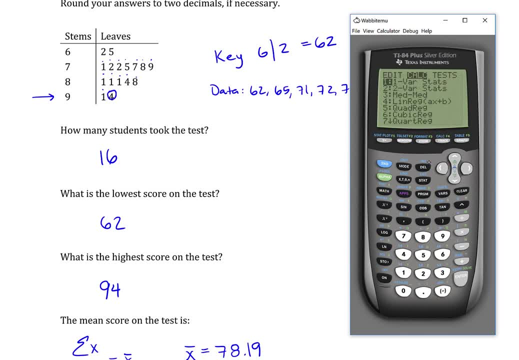 Another common option is if you hit Stat and then come over to Calc and 1-Var Stats. this is what's called Single Variable Statistics, And it will do a bunch of different calculations on a set of data all at once. If you just need a single statistic, 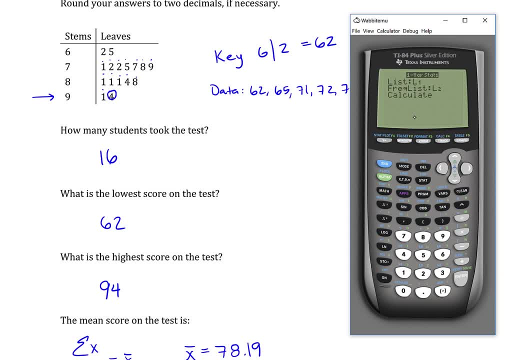 it doesn't save any time, But if you have a bunch of statistics then it is a time saver. The list where your data is, the frequency list, is a different thing, where, if you have a list of values that tell you how many times each data item exists, 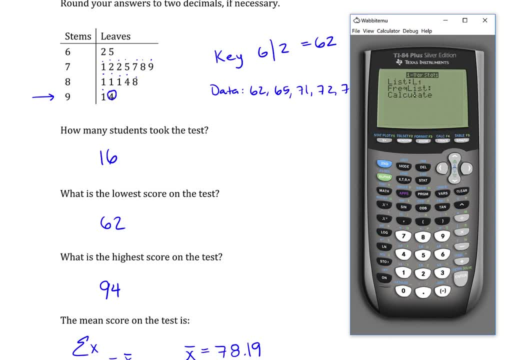 We don't have that in this case, so we'll just leave it blank. Oh, and if you're not seeing this menu at all, that's okay too. You're just going to hit 2nd and 1 after the 1-Var Stats function comes up. 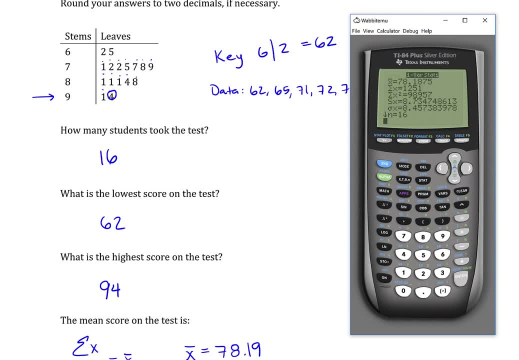 and then press Enter. It's the same effect. It's just a way that the calculator kind of does menus for the later model calculators. But at the top X bar you'll see that it has come up as 78.19.. 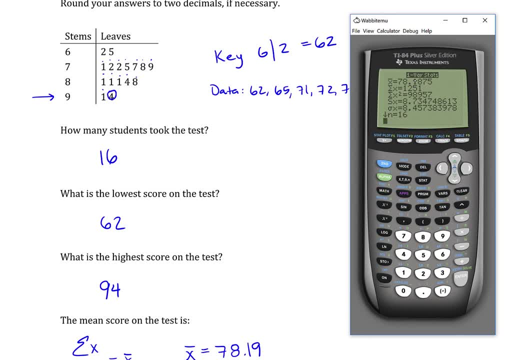 So lots of different ways of achieving this. Choose whatever is most comfortable for you.